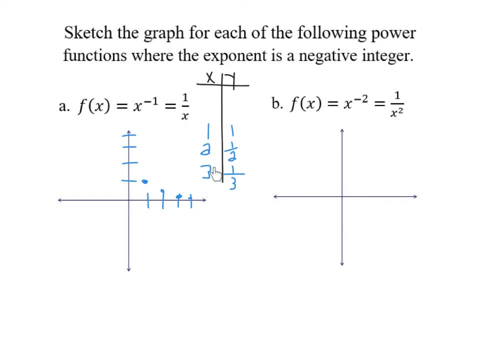 Because you're never going to end up. You're never going to end up with a negative value by plugging in positive numbers here. As we look at values between 0 and 1,, of course, taking their reciprocals gives us larger and larger y values. 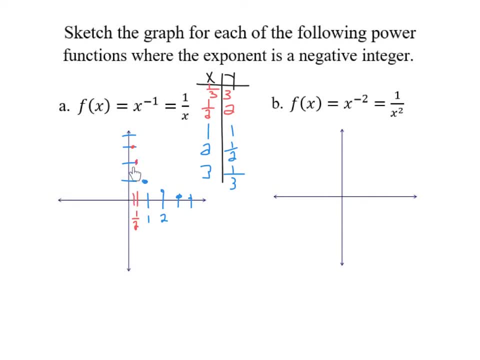 So we're going to have the point what, 1 half and 2, and then 1 third and 3, and those values keep getting closer and closer to the y-axis as our x values get closer and closer to 0,. 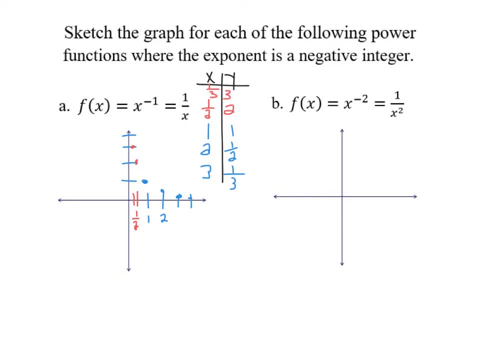 but they just keep going up. So it looks pretty clear that we have a curve that does this. Pardon the waviness of the line, but you can see the basic shape here. right Now, of course, when we plug 0 in, we have 1 over 0, and that is undefined. 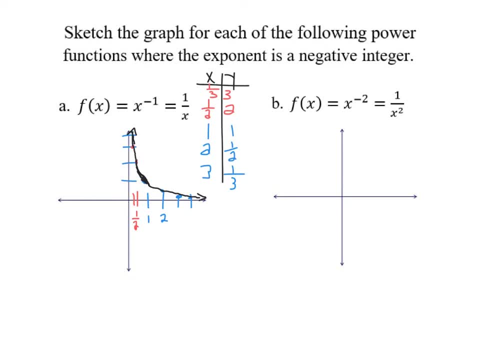 so we're not even going to plot a point there. And then when we plug in negative values here, right, we're going to basically have the same thing happening, just for negative. So negative fractions like 1, half are going to be negative 2, you know. 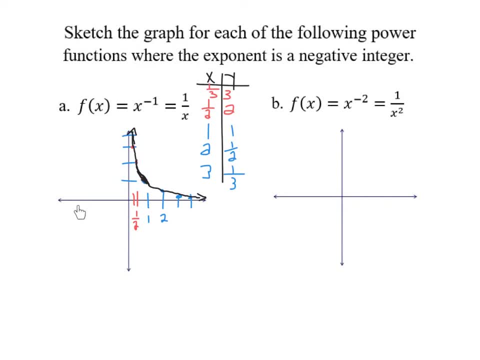 and as we go out to like negative 2 and negative 3, we're going to be plotting like points that are close to the x-axis again with their reciprocals. So it should look something like this: 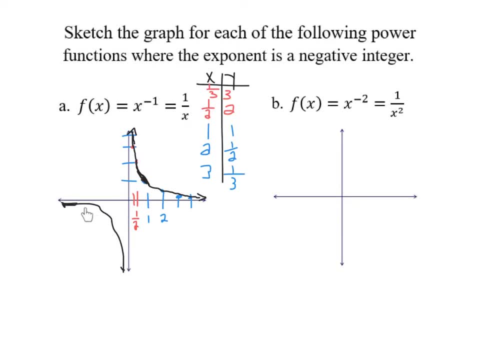 Okay, you get the basic idea, except for the waviness of the line, And the graph that we have here is what we would call the basic hyperbola. That's essentially what we have here, where we do have a vertical asymptote at 0,. 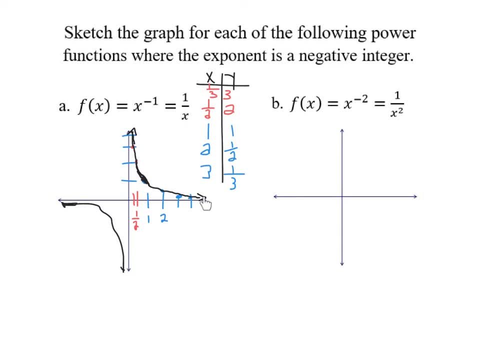 at x equal to 0, and we also have this horizontal asymptote of y equal to 0.. All right, so what is it going to look like if we have x to the negative 2, where, when we plug in our numbers, 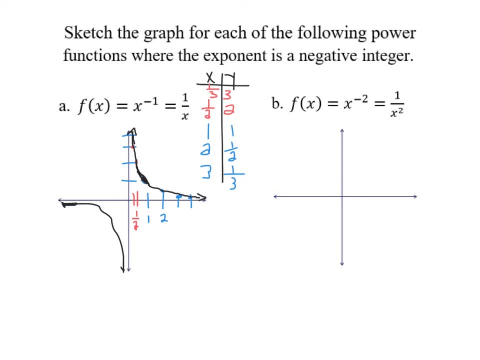 we're squaring them first before we take the reciprocal. If you think about it, it's not going to change things too much. I mean, when you plug in 1, you're going to get back 1 still. If you plug in 2, you'll just have 1 over 2 squared. so 1. fourth, 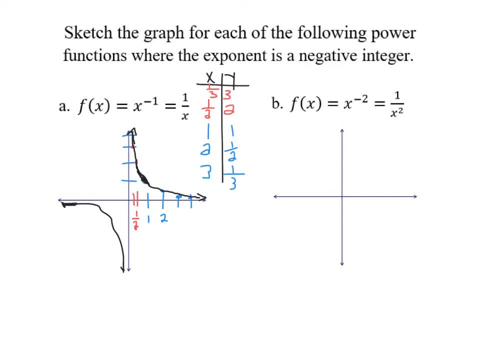 and 3, 1 over 3 squared, which would be 1 ninth. So you're still going to have these small y values. when you're plugging in whole numbers and when you do the fractions, you're basically going to. 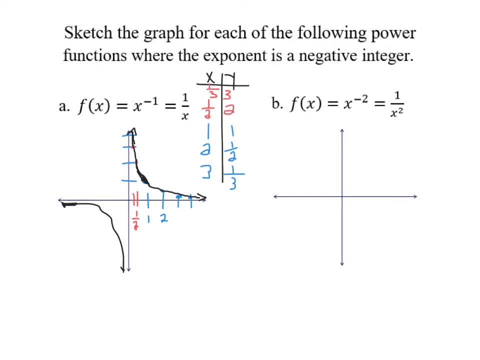 uh, have the same thing happening where you're getting bigger whole numbers, right. So if I plug in 1 half, I'm going to square that I get 1 over 1 fourth, which will flip it and become 4.. 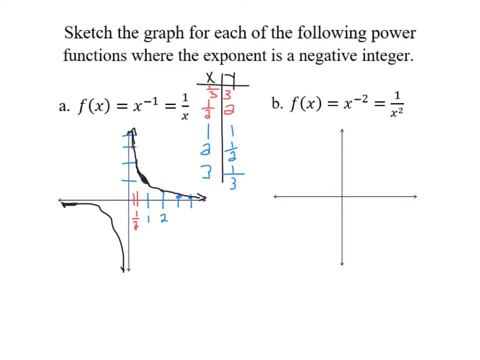 So we're essentially going to have the same thing happening for positive values Now when we um go to the negative side of this. we're basically going to have the same kind of thing happening, except now all these values that were negative before are going to get squared and become positive, right. 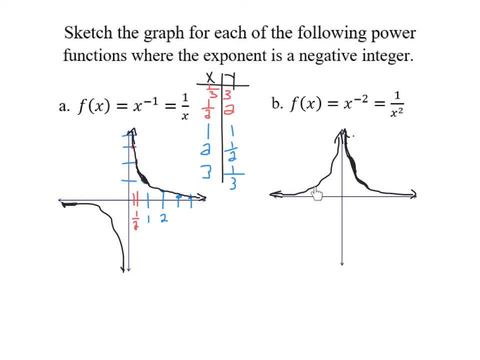 So the curve will look like this and it will actually be symmetric, right? Because if I plug in positive 2, I'm going to get 1 fourth. If I plug in negative 2, I should get back 1 fourth. 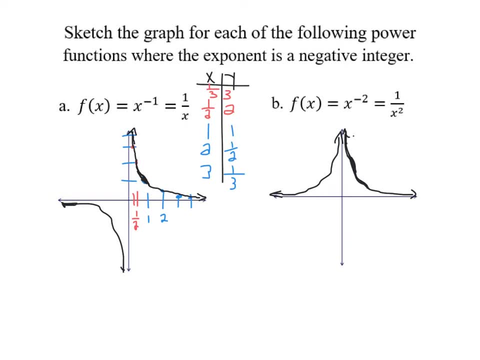 So we're going to get back the same y value whether we plug in a positive or a negative. All right, So this is the basic pattern of these graphs, where the exponent is negative on a power function. So let's quickly, um, take a look at other ones. 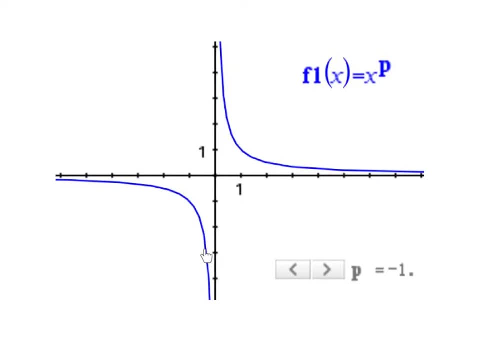 Just to verify what we did, we can see, this is: uh, this is here's the basic hyperbola that we were getting when p was negative 1.. And here all our values are being squared. We've got p to be negative 2, and there's the graph we were sketching. 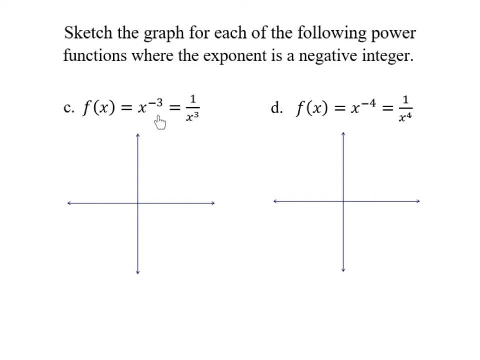 So what do you think is going to happen when we go back to a, to an odd exponent, something like x, to the negative 3?? Well, I'll give you a choice. It's going to be like one of the two graphs we saw before. 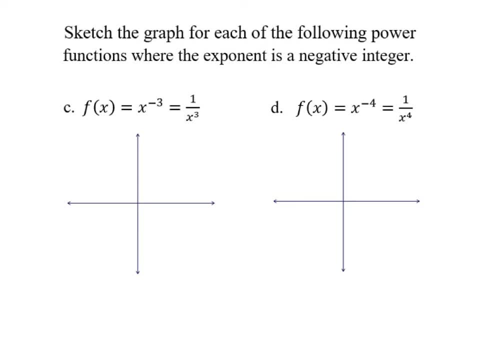 So which one do you think it'll be like The x to the negative 1? Or the x to the negative 2?? Well, hopefully you didn't have to think too long of that. Yes, it's going to be like x to the negative 1, the other odd one. 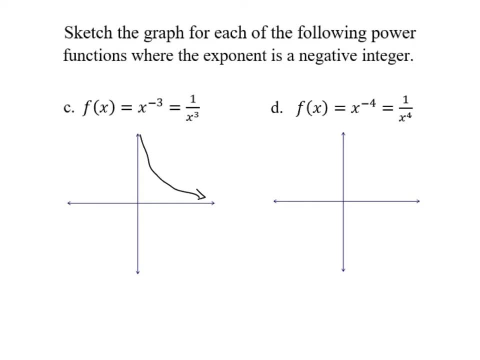 So so our graph here is just going to- uh, that was not a very good graph there, but it's just basically going to mimic what we did for x to the negative 1. It, it, it actually is a little steeper. 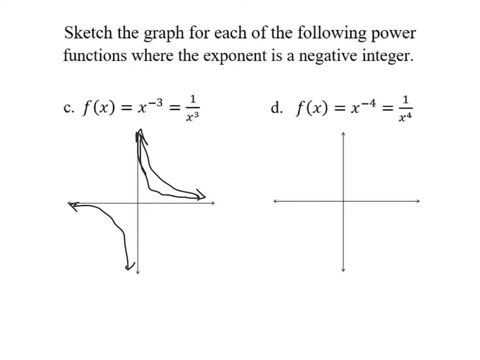 Like it's going to. it's going to go up a little faster and come down a little faster, but we're not really worried about that. It was mostly the g. The general shape is what we're looking at. And then, of course, x to the negative 4 is going to make sure that all the output values are positive. 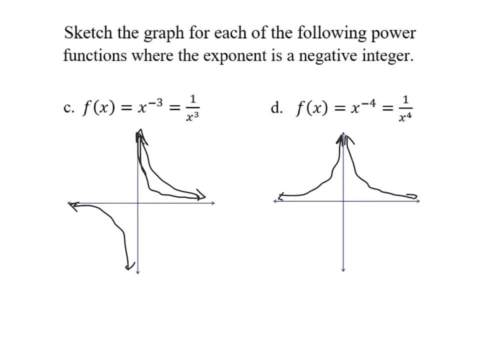 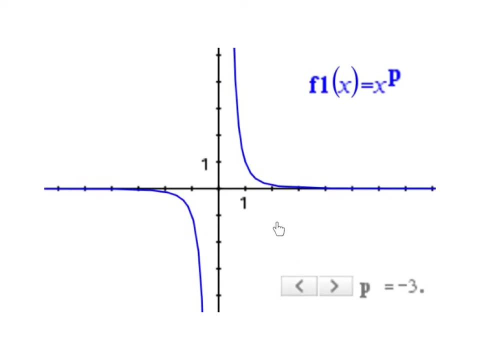 So it's got a curve that looks like this. Here's our check on what we just sketched with: uh, our exponent being negative 3.. It looks a lot like when it's negative 1.. And here it is: when it's an even negative, like negative 4, it looks a lot like negative 2.. 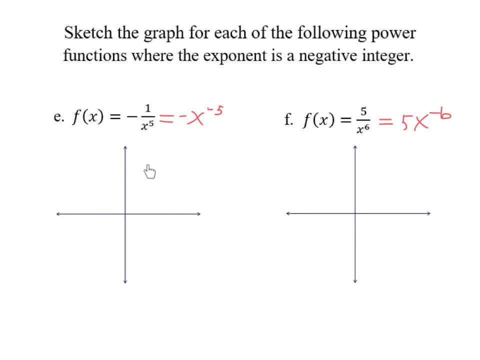 So now we've established the pattern with the uh, even and odd negative exponents, what those graphs look like. Now we're going to throw into it. you know what, if we have, uh, some coefficient in front, that's either negative or positive, what's that going to do to the graph? 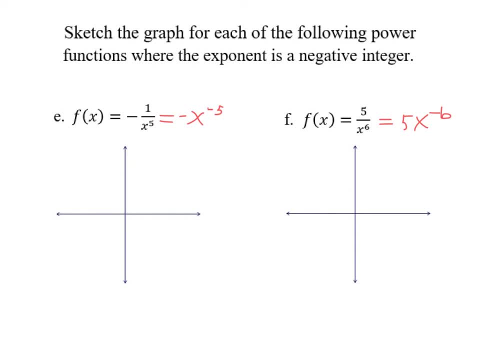 So I've rewritten it so you can still see it is a power function right on both of these. Um, so why don't you, uh, pause the video and sketch what you think this graph will look like? Don't worry about any specific points, but just the general shape. 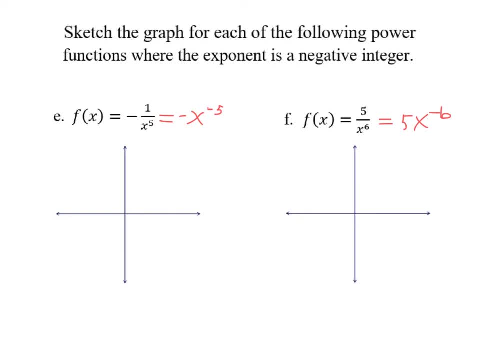 All right, see if this is what you got for letter E. Hopefully you didn't sketch this red graph. This is what it would have been, had it, of course, been a positive x to the 5th. So if it's negative, it's going to look like this: 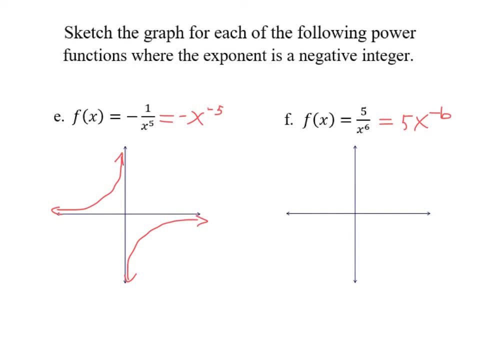 Yes, the negative just reflects the graph, right, What was up here now gets reflected over the horizontal axis, becomes negative, And what was negative before becomes positive and it's up there, All right. uh, perhaps you went ahead And also did. uh, the next one with x to the 6th. 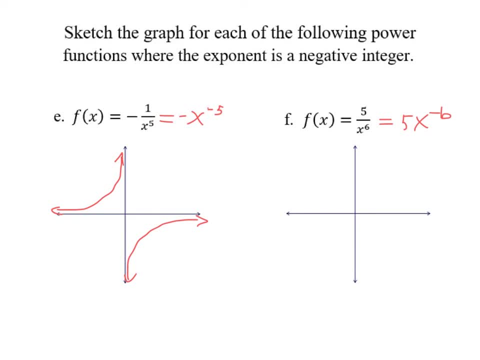 Let's think about it. It's got an even exponent, so an even negative exponent. So normally we would expect it to, you know, be doing this thing right where we're up here. But because, let's see, and with a positive coefficient in front of it, that's not negative, it's going to stay that way, right. 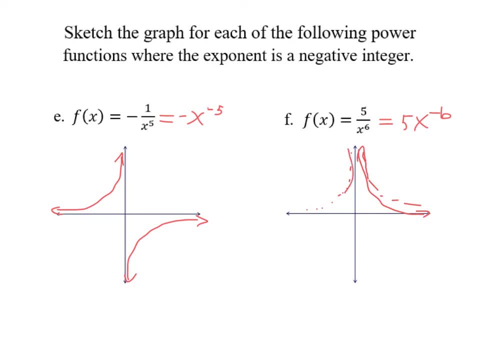 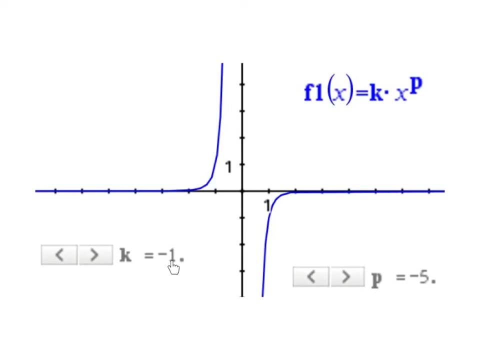 So so we'll just go with. go with this curve. I'm trying to keep it looking right. All right, Not quite right there. It's supposed to be getting closer to the y-axis, All right. Here's a look on the calculator when um, the exponent's an odd negative, but we also have a negative coefficient.